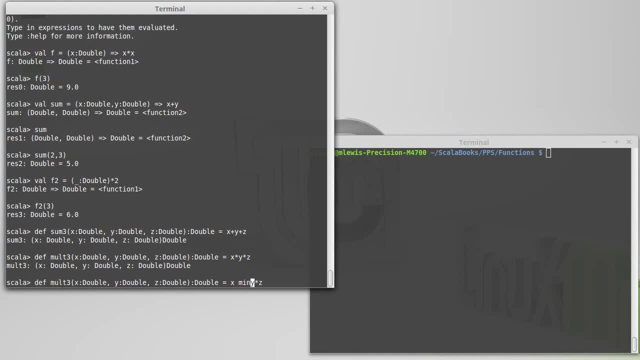 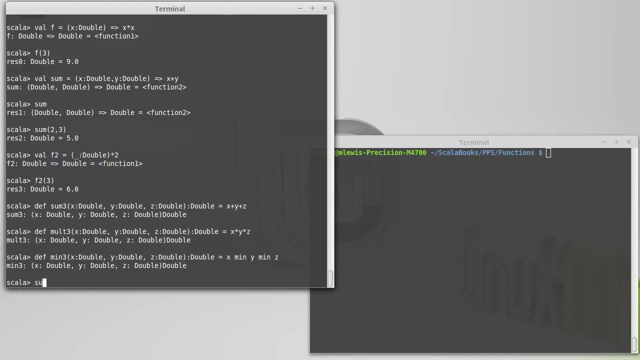 Other ways that I could combine them. Well, maybe I want the minimum value of these three numbers, in which case then I could use min as an operator And do that, And we can show that all of these work. Sum of 1,, 2,, 3.. 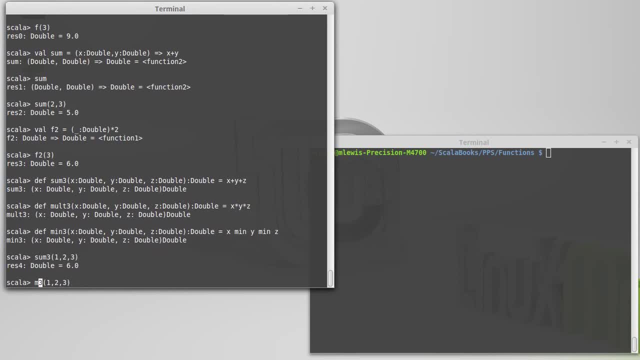 Sum of 1, 2, 3 gives us 6, mult- I'm going to go ahead. and 4, 2, 3, gives us 24, min gives us back the 2. I can very easily define a max. 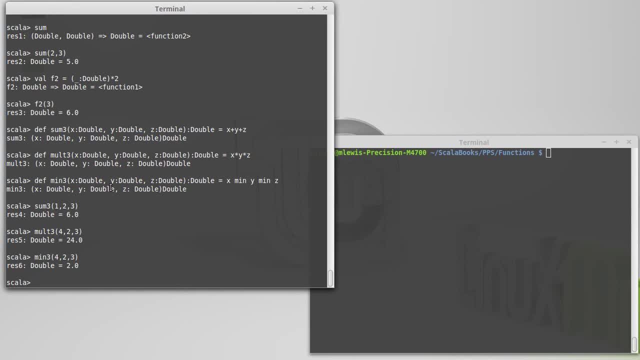 What I'd like to do is I'd like to take all of these functions, and possibly others, and combine them into one single function, And I want to call it. instead of calling it something like sum3,, I want to call it. 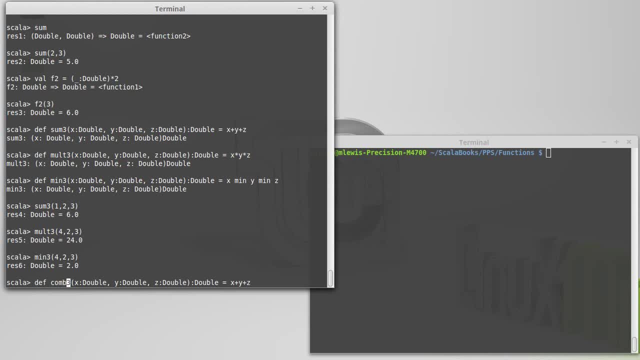 Combine3, because we're going to make the way in which we combine them be unspecified. The user gets to specify how we combine them so that all three of these, So they can call it one way and get a sum, call it a different way and get a product, call it another way and get the minimum. 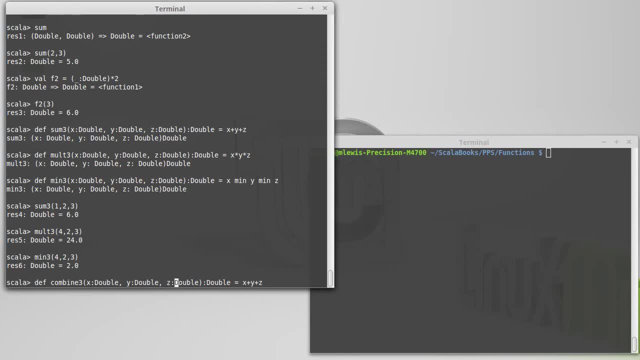 So, in addition to these three value arguments, I also need the function that I'm going to use to combine them, And we'll call this function f. Now, just like these others, we have to specify a type here, And so it turns out the way that you write function types in Scala uses that same rocket notation. 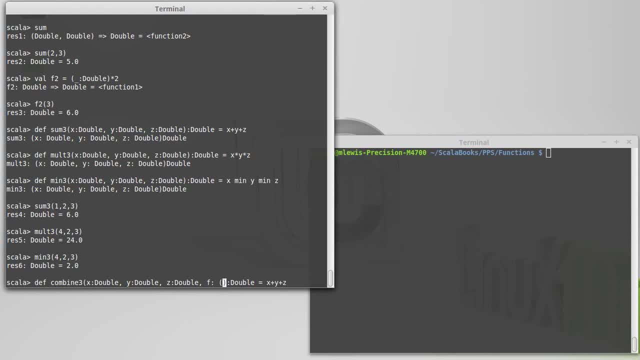 And we start off with the arguments, So the inputs to f. f could be a plus, in which case it takes two arguments, an x and a y, And it gives us back another value, Which is the sum of the two, And we're going to do that. 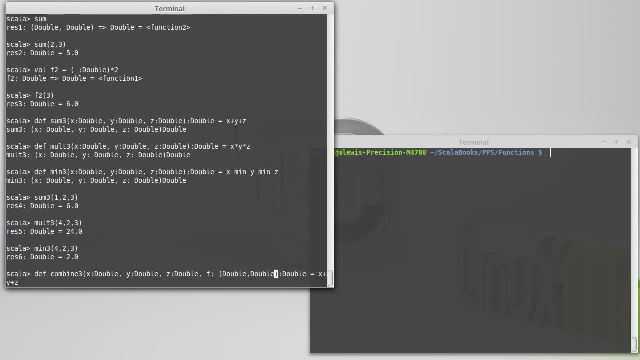 The sum of those two And since our inputs are doubles for the whole function over here, The inputs to this function will be doubles And it will produce a double. So this is how we write the type a function that takes two doubles and gives us back a double. 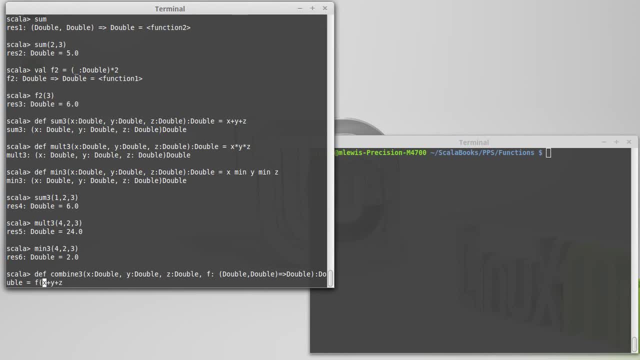 And then, instead of putting the plus here, I can call f on x and y And take the result of that and combine it using f with z, And so this will actually do the proper precedence as well, Assuming that this operator is left associative. 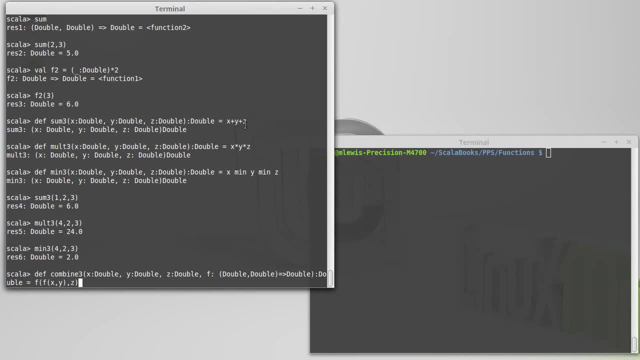 So here, this is really x plus y, And then that result plus z. That's what this will do. It takes f and combines x and y, And it takes that result and combines it with z. Now, the power here is the fact that I just wrote this one function. 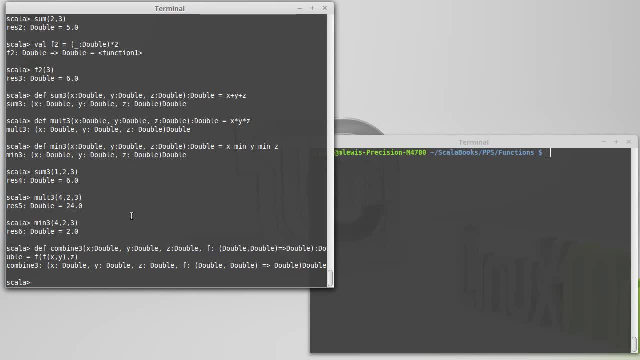 And it's supposed to do what these three functions did, As well as possibly other functions, Other things that we haven't come up with yet. Any way that I wanted to combine these three numbers, As long as I want it to be left associative- 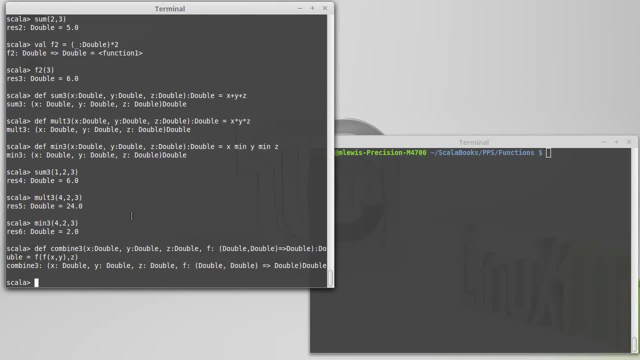 And I want to use the same operator between them. I can do that with this function. We can demonstrate that. So let's go back to our one, two, three, And I want to add them. Well, I pass in a function. 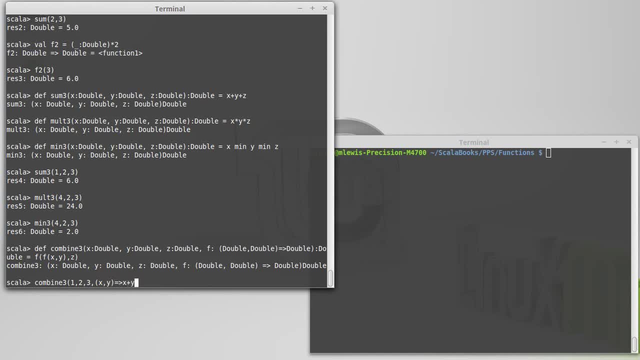 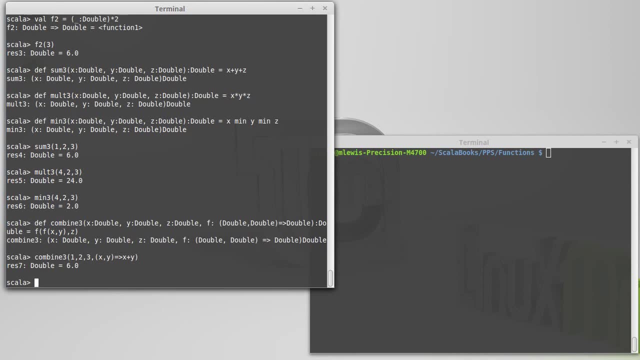 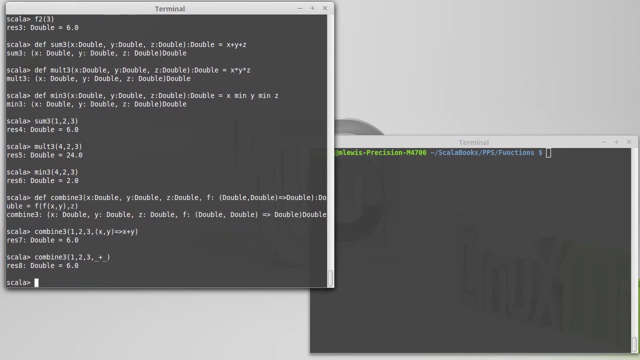 Okay, That represents addition. So x and y is the input: Rocket x plus y. This is one of those perfect places to use the underscore, though, Because I can also write a lambda expression for addition: That is something plus something. Turns out that these two are equivalent. 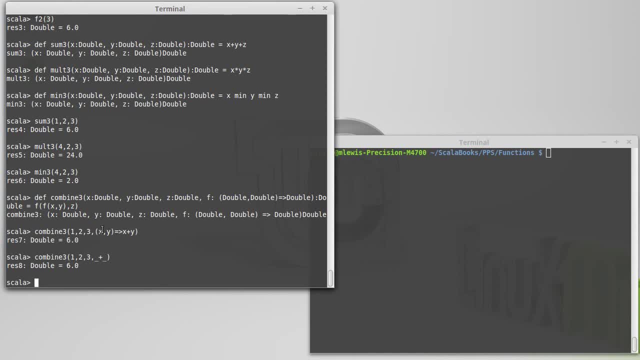 You can't always use the underscore notation, And you should remember how to use the rocket notation, Because you'll always be able to fall back on it. But there are situations like this where the underscore notation is just far more succinct And I would argue it's actually very highly readable as well. 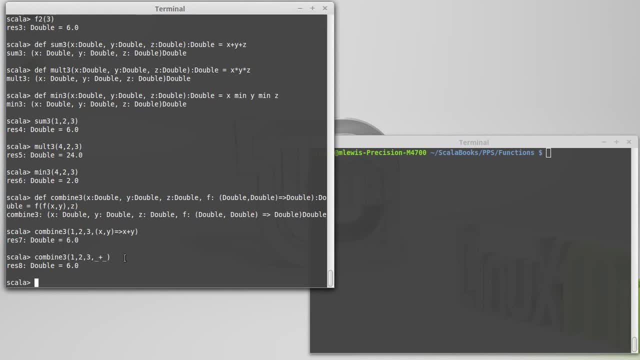 Because I'm combining one, two and three with something plus something, As opposed to having the x's and y's getting in the way there. What if I want to multiply the three And we'll go ahead and change this back up to a four, as we had done before?